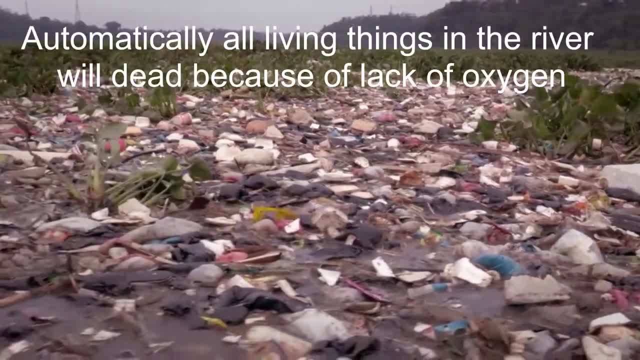 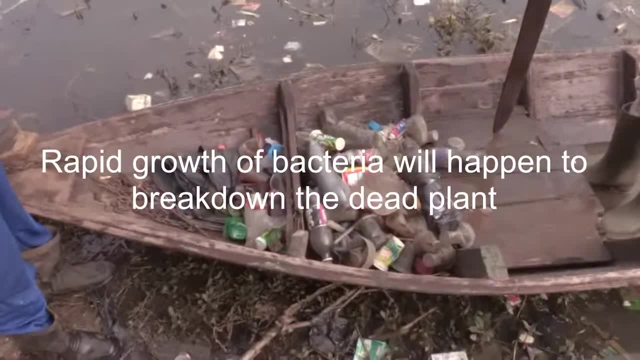 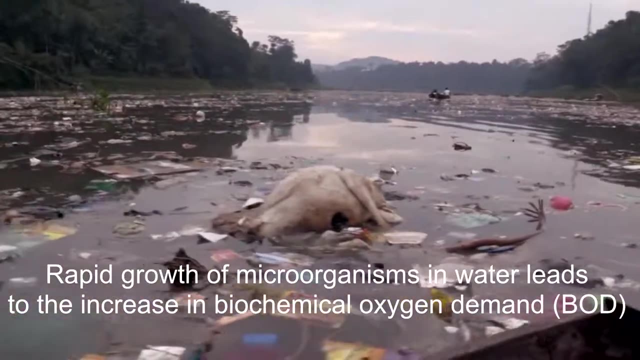 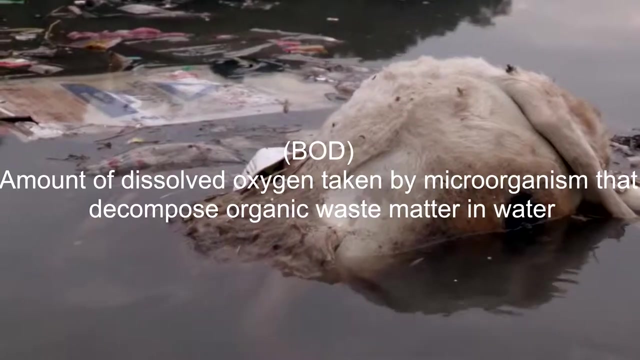 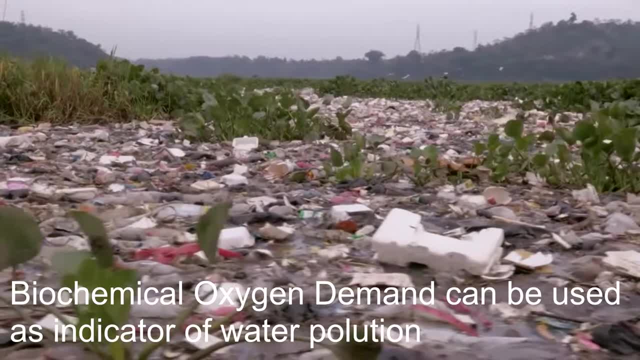 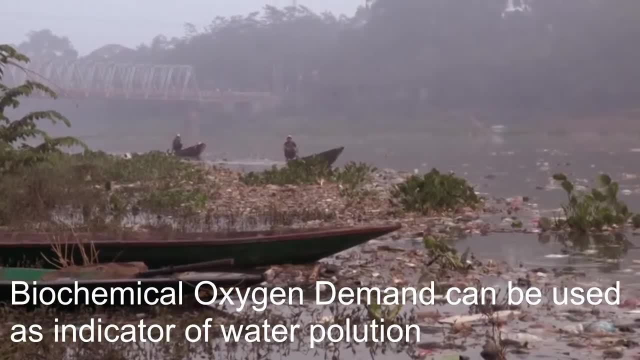 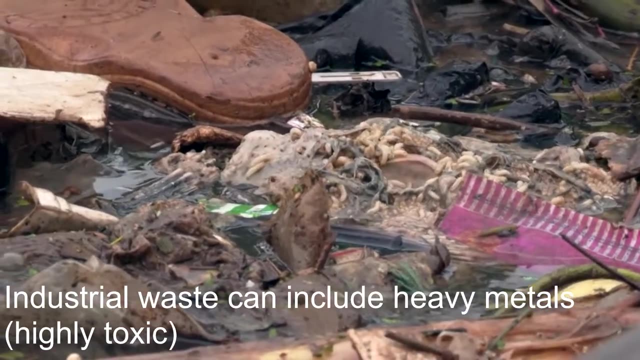 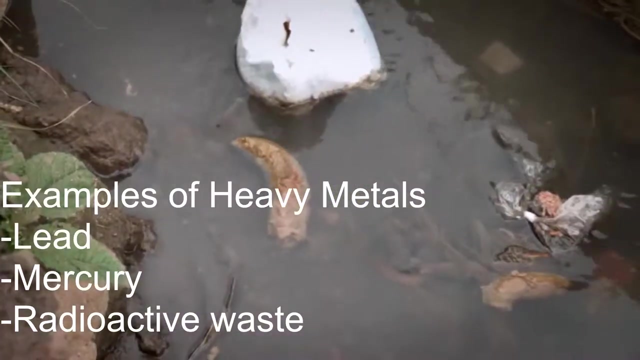 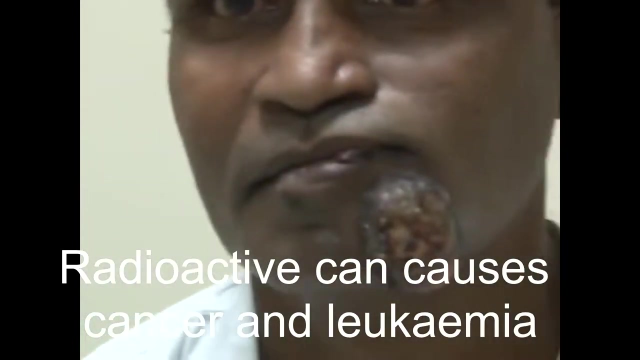 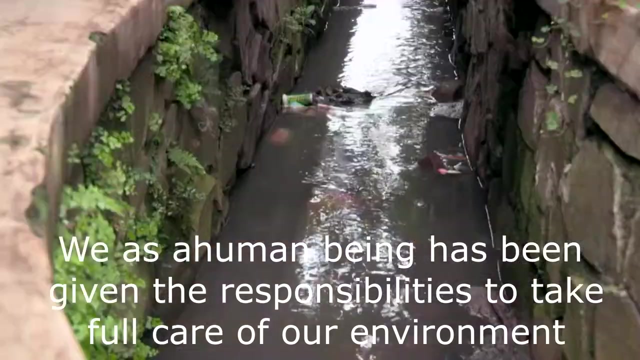 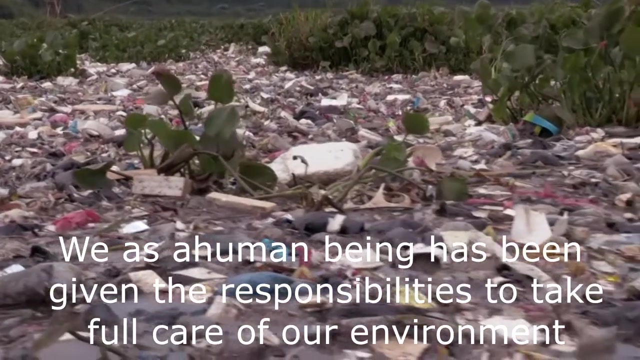 Biochemical oxygen demand can be used as indicator of water pollution. Industrial waste can include heavy metals. highly toxic Examples of heavy metals: lead, mercury, radioactive waste. Radioactive can cause a storm, Cancer and leukemia. We, as a human being, has been given the responsibilities to take full care of our environment. 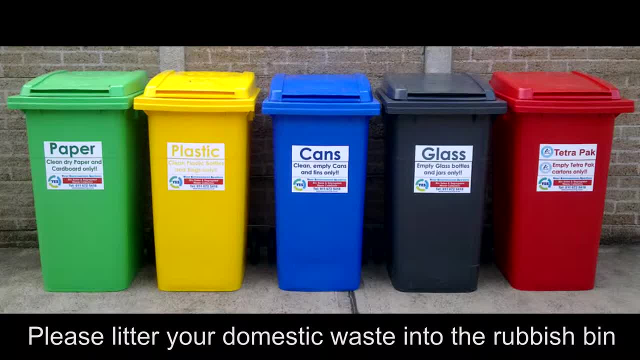 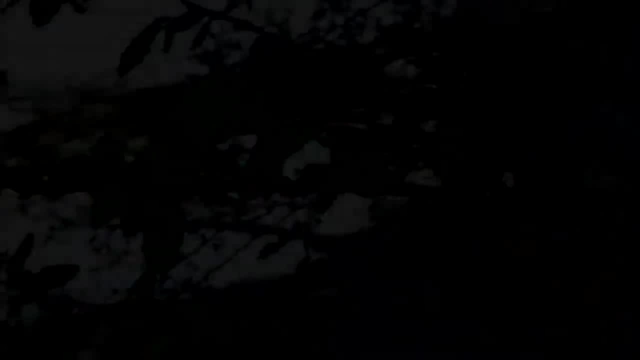 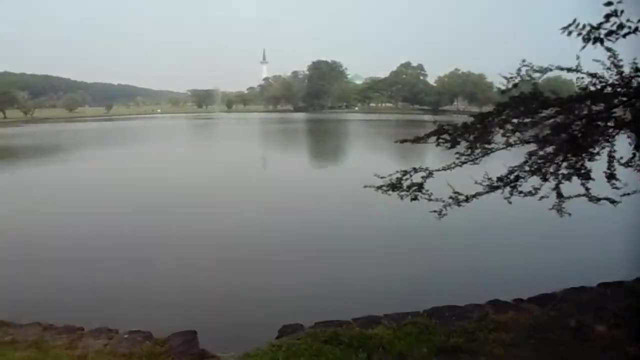 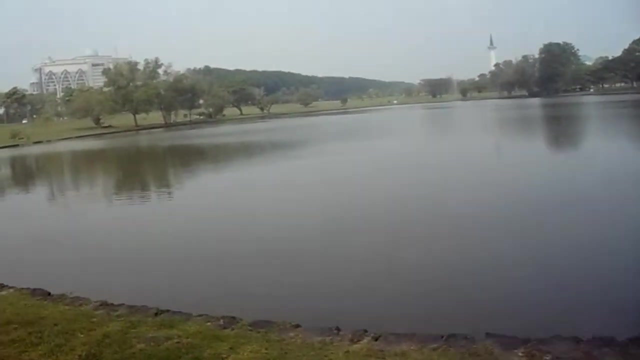 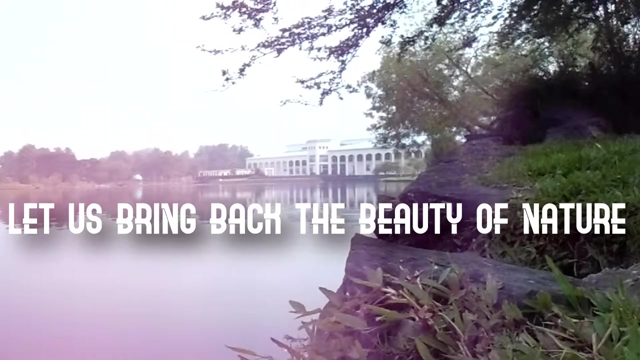 Please litter your domestic waste into the rubbish bin. At least the water pollution activities can be decreased. Let us bring back that beauty of nature, Be grateful to what God's given to us. 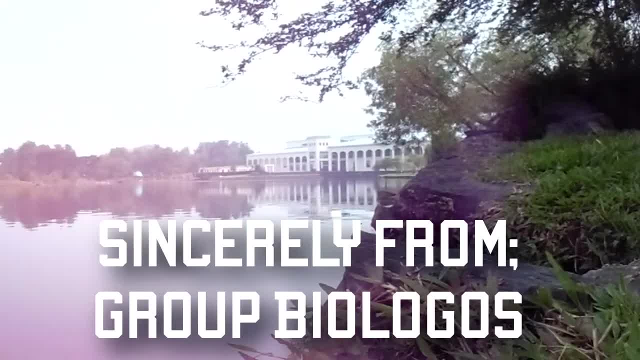 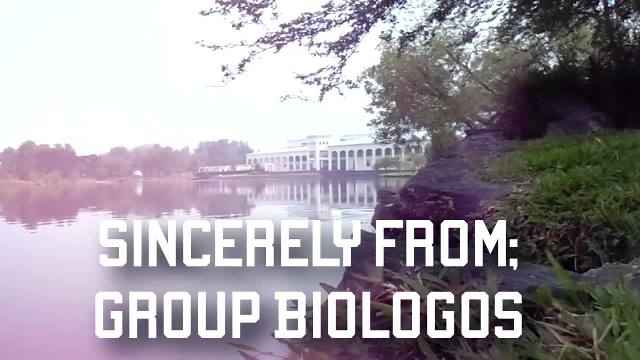 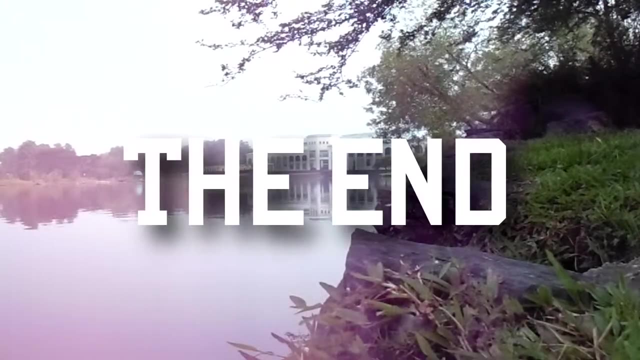 Sincerely from Group Biologos The End © transcript: Emily Beynon.